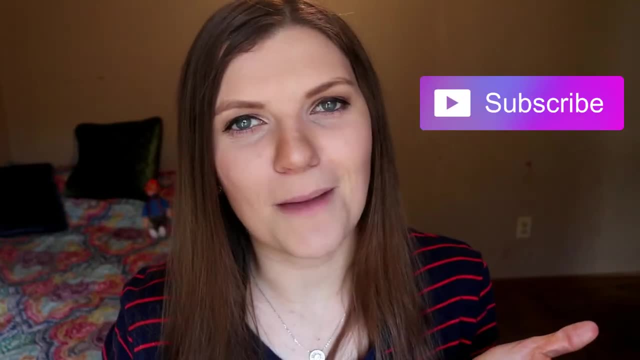 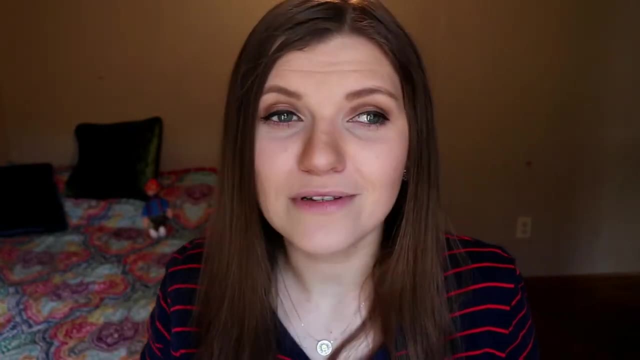 So if you're new here, go ahead and subscribe so you can see every time I post a new video. I'm usually doing craft projects or some type of customized stuff sometimes, where I'm doing custom labels or gifts or games. So go ahead and subscribe so you can see every time I post a new video. 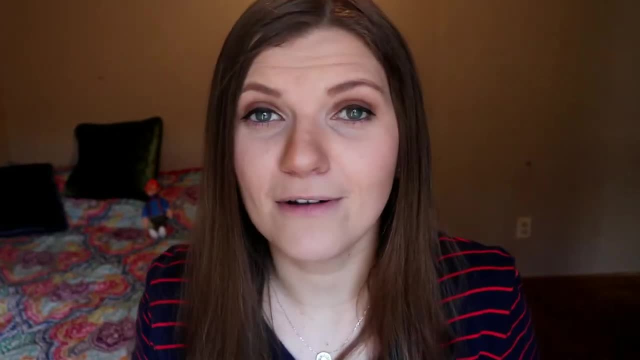 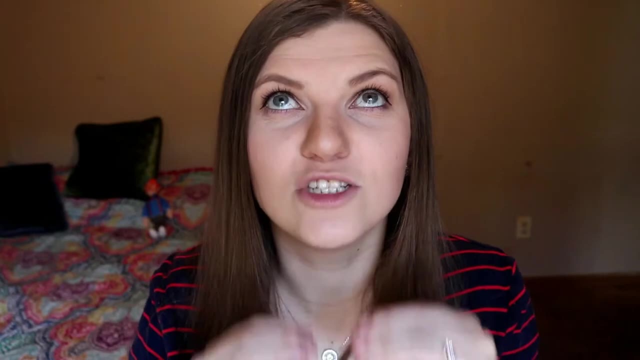 Don't forget to hit the notification bell so you're notified every time I post, because sometimes just being subscribed is not enough. I hope you guys like how this game turned out. I promise you you won't regret it if you do this. It's gonna be super, super fun. So let's go see how to make a customized, personalized guess-who. 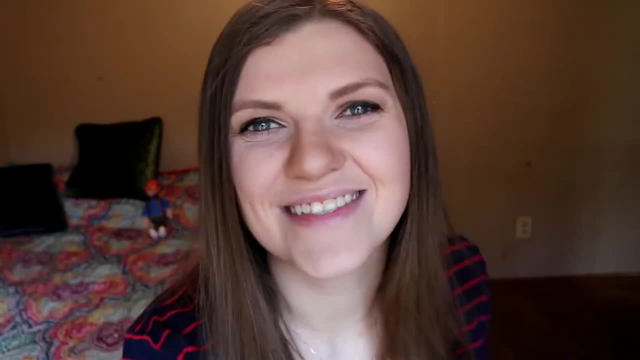 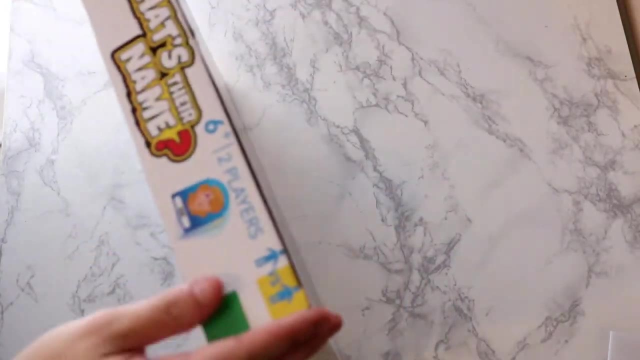 specific to you, your friends and or family. Let's go. We're gonna start with a game of guess-who. I got this at the dollar store, at the Dollar General, for $5.. I highly suggest Going to Walmart and paying a couple dollars more and getting the actual guess-who game, because these boards were made kind of cheap. 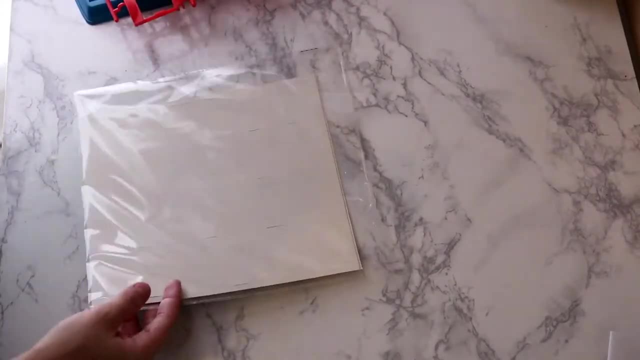 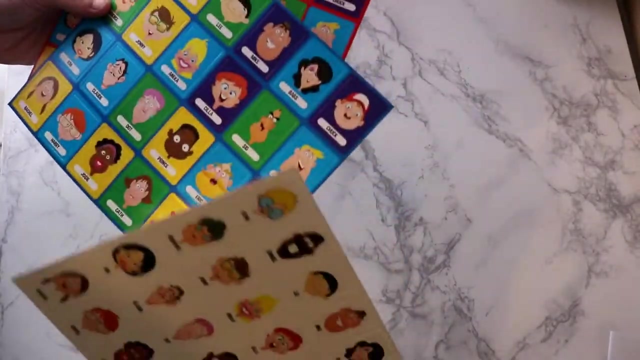 But if you're going the cheap route, the Dollar General, five bucks. That's where I've got this. I'm gonna put everything aside for now, because my main focus is going to be these images. These are the cards that you put into the boards and that you draw from. 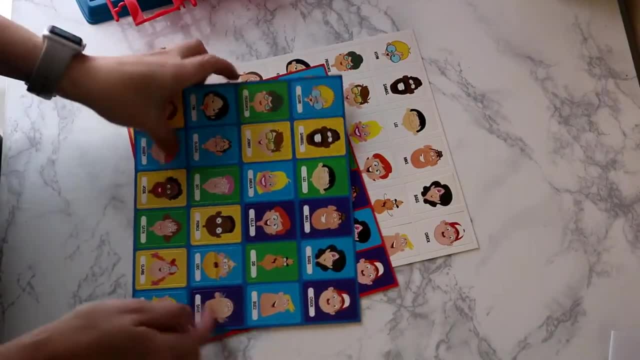 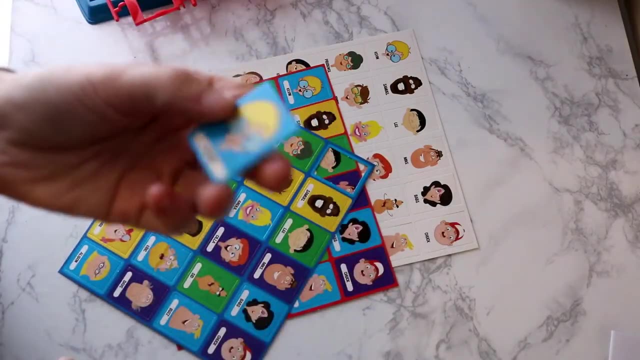 to figure out what character you're going to be guessing of, And I'm actually just going to use these original cards as a template so I can figure out how big of a size I need to size my specific images to. So what I'm going to do is I'm going to just pop out one of these cards. 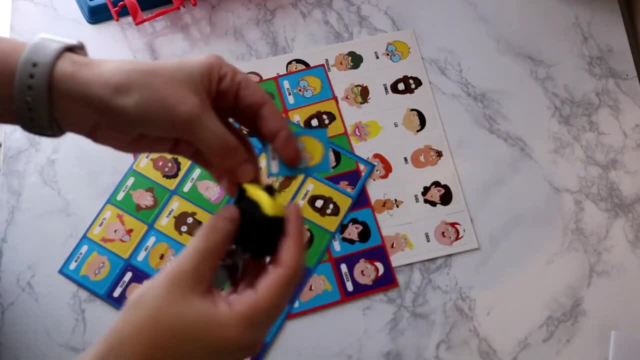 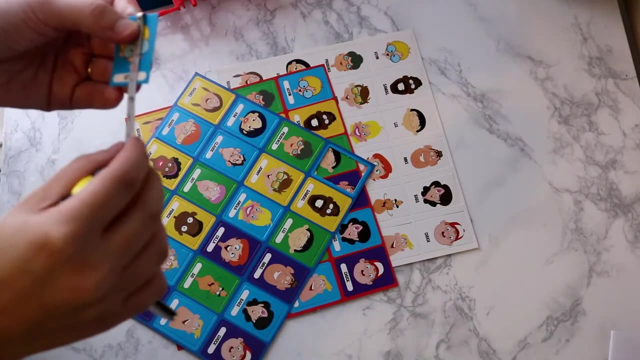 We don't need to pop them all out because we don't need them. And I'm gonna take a tape measure and I'm just gonna measure how big across and how tall this little image is, So I can refer back to that when I am making my pictures. 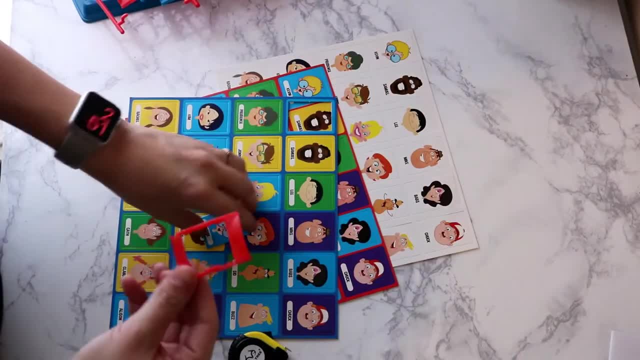 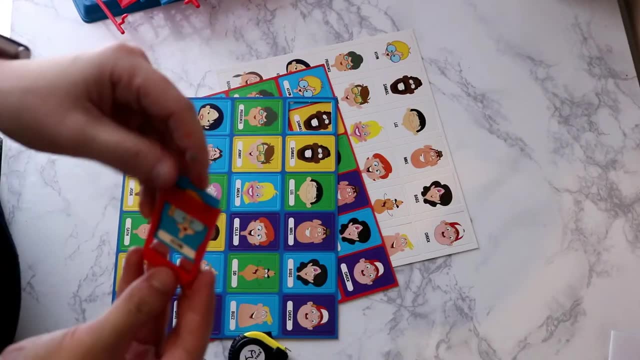 Keep in mind: if you're using the guess-who brand or a different brand game, your images size may vary. So just measure the cards and, whatever game you have, the cards that come with it, so you can find out the exact size you need. 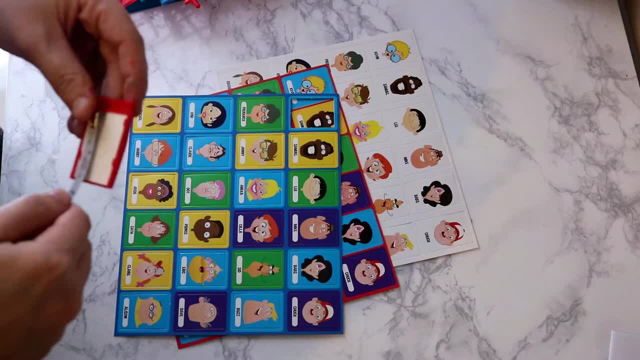 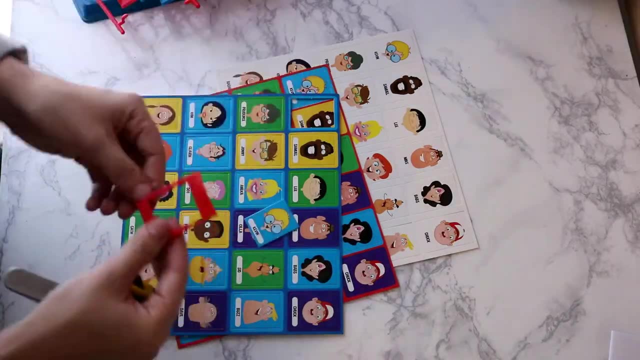 I did decide to put this inside of one of the little pieces That it will slide into to remeasure again, just to see if I have a little wiggle room with the sizing and the measurements. Next, I'm going to pop out all these little plastic pieces that the cards are going to go into and I'm going to snap them onto. 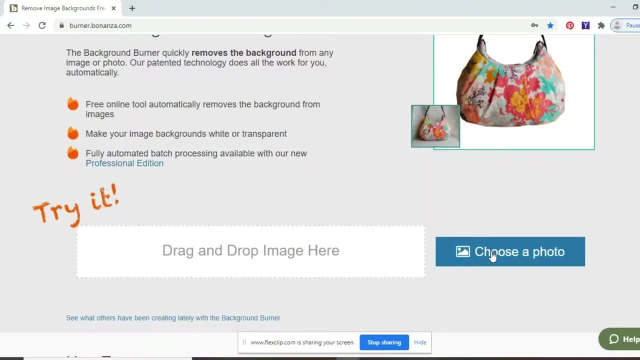 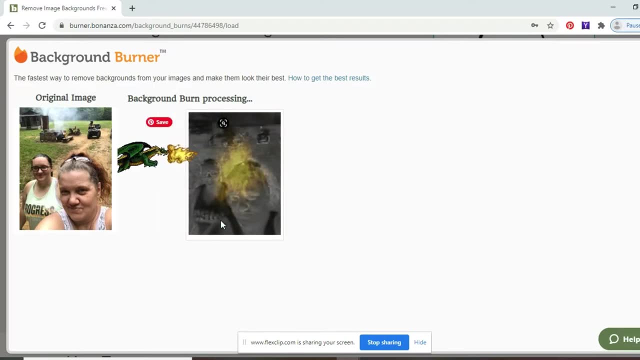 the board where they go. So it's ready for when I get done with printing my images. Now, to show you how I take the backgrounds off my images, I go to this burnerbananzacom. I just Google background burner. It's one of the first searches that comes up and this is just an easy way to remove backgrounds. 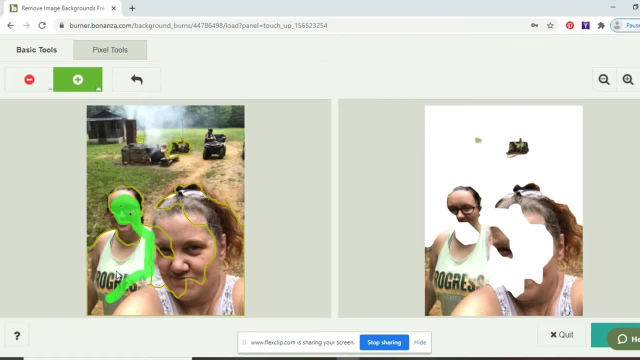 I'm gonna kind of do it really sloppily. just to give you a rough idea. I myself prefer to put the images on my iPad and remove the backgrounds on Procreate. It just works best for me. but if you don't have an iPad Pro and a Procreate, this is a really good way to do it. 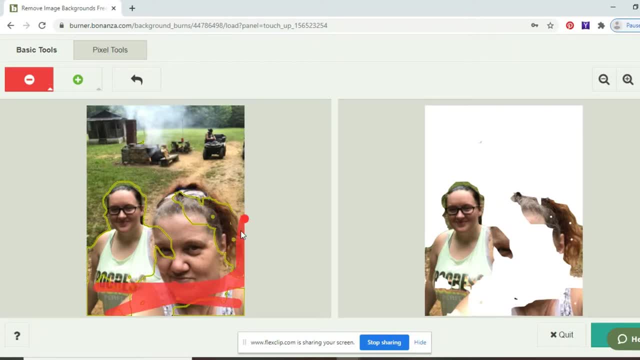 It's just gonna take some time. You just got to sit and piddle with it. I've done a really bad job here. just as an example to show you how easy the background burner can take your background off and you can use the little red dot. 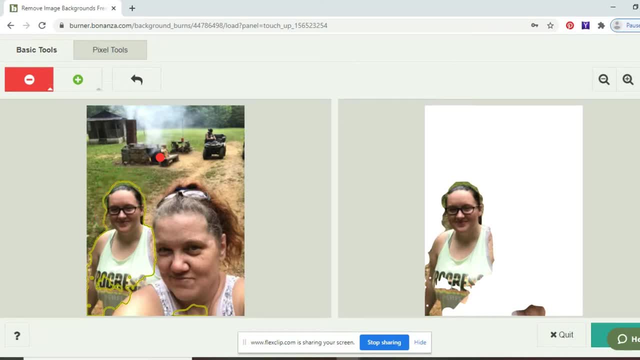 to erase background and use the green to put things back. But again, spend a little more time on it and it'll probably turn out a lot better for you. Next I'm going to go to Canva. You guys know I love Canva- It is free. 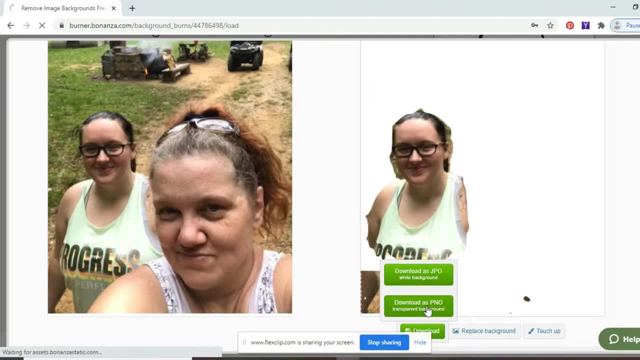 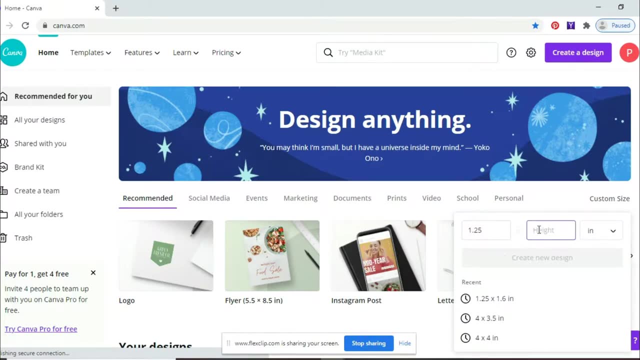 You might have to make an account, but I use a free account. I don't use a paid account. I'm gonna go to a custom size and I'm going to put in the size of the cards that I'm going to make. This again may vary based on what size cards for your specific game board. 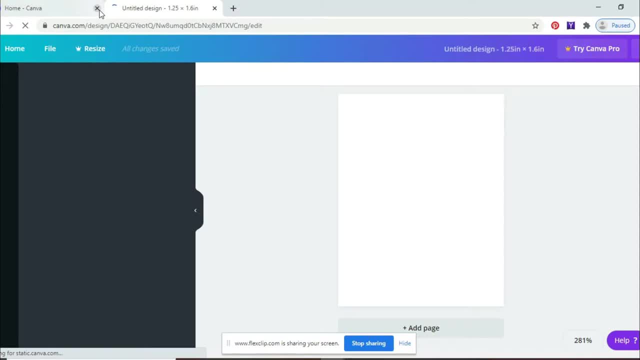 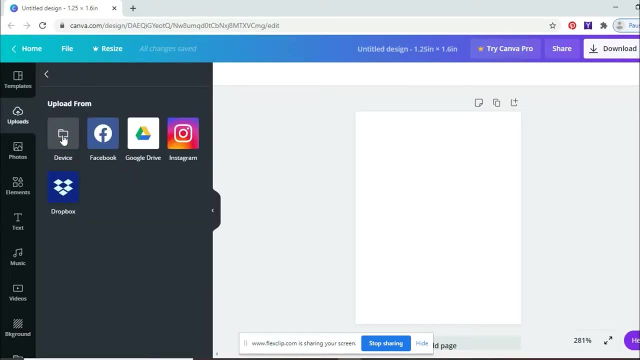 Mine are going to be 1.25 inches by 1.6 inches. Now that I have my basic card template pulled up, I'm gonna sit and make all of my individual pieces for all of my characters or my people in the game. 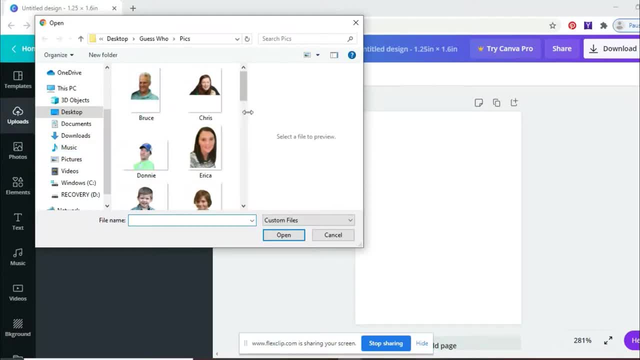 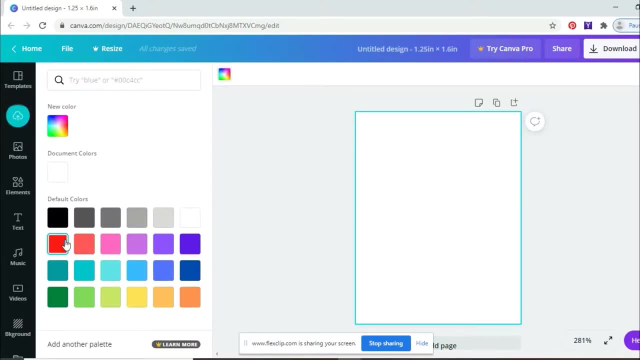 I'm going to add the picture on there that I'm going to use for the character and I'm just going to pretty much make my card. You can make these however you want. I did decide to do a red background, a blue background for the cards in the boards. 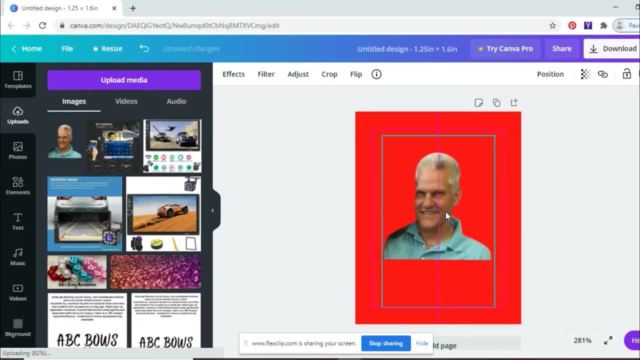 and then I did a separate white background of the same exact image for the cards you draw out of. So first thing I did was just make my first one, and once you get that done, you can again make this however you want. I just repeated the same process, changing out the pictures and names. 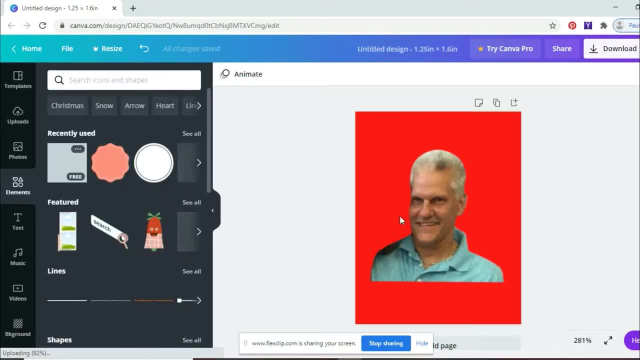 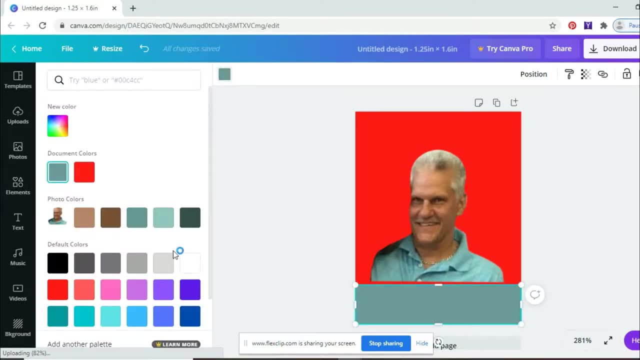 I did put a white rectangle for the name because I wanted it to be easily readable And if you didn't see how I did it before, when you add the image, you just click on uploads. It's the second option down on the left and that's how you add the image. 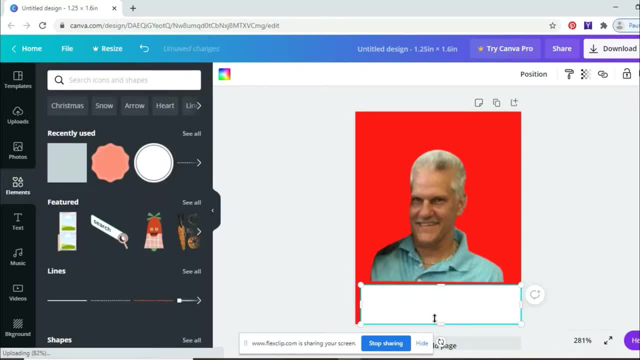 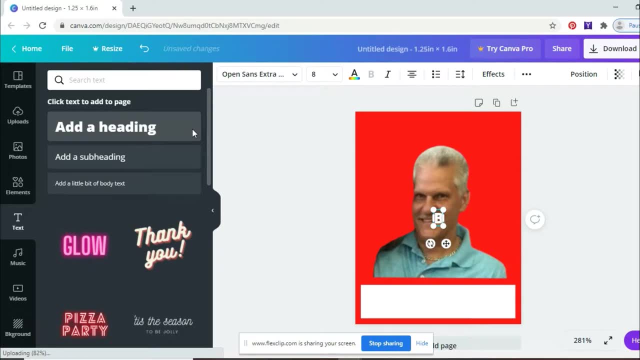 Elements is how you add the rectangles or any other shapes, And then, of course, you just click text and you can choose whatever font you want to add your text and to change the color of the text or the shape. you just click on them and you can change the color that way. 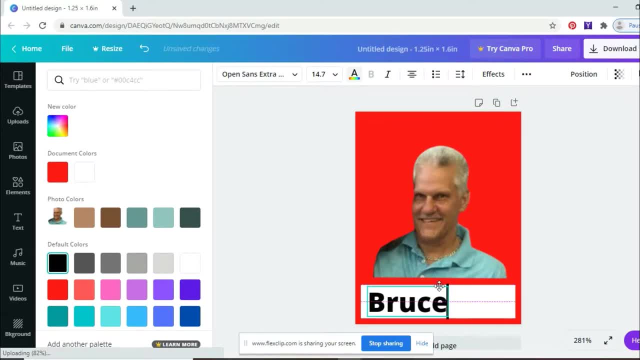 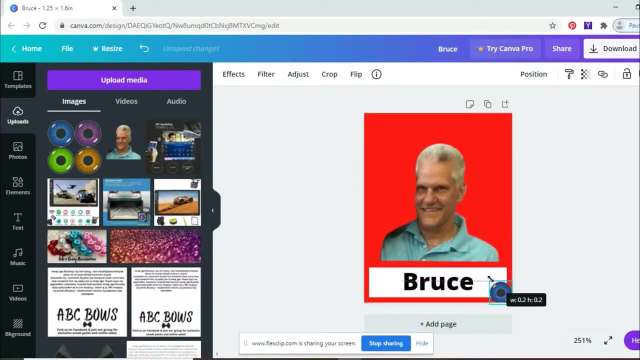 Also, Google searched an eye clip art so I can add the eye color of everyone onto their cards, just to make it easier, because in the real-life pictures like this you can't exactly tell their eye color. great, So I did decide to do that, just to add a little bit of extra. 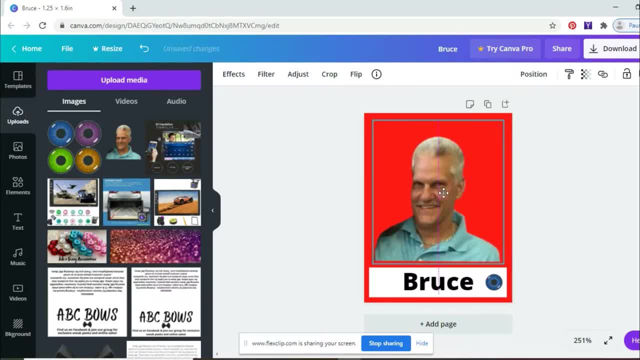 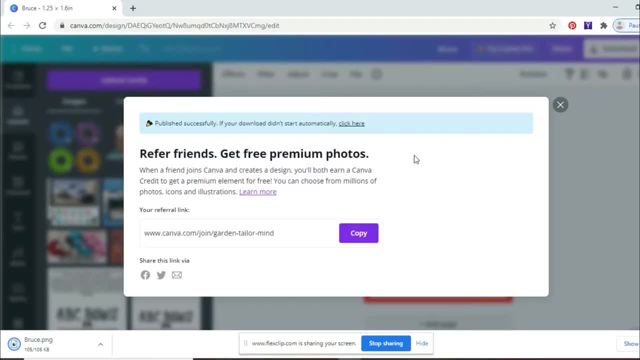 easiness to the game. Does that make sense To make it a little easier? because just you want to be able to see their eye color. Once I got this image how I wanted it, I downloaded a copy of it, a PNG or a JPEG, whichever one works. 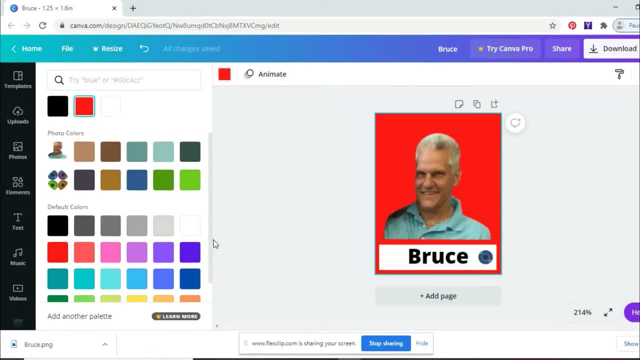 And once I downloaded the copy I changed the background and to do that I clicked on the background and then you just pick whatever color you want, And then I redownloaded it again in blue and then I took the background again and made it. 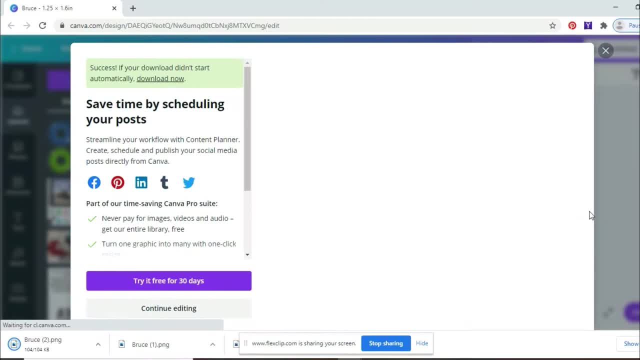 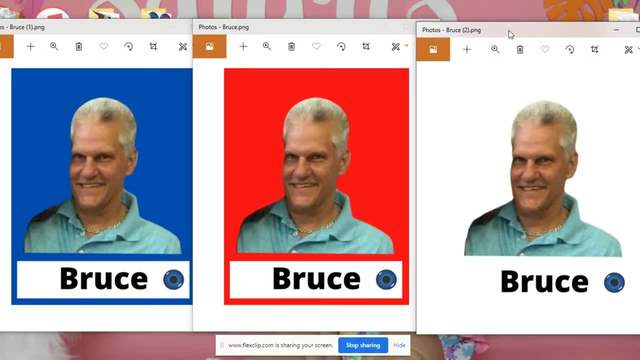 white for the card that you draw, because, again, I wanted to have them all three different and I did this for every single character. So you have a blue, a red and a white. Now all I did was take those same images and take out the name and the image of the person and change it out for the next. 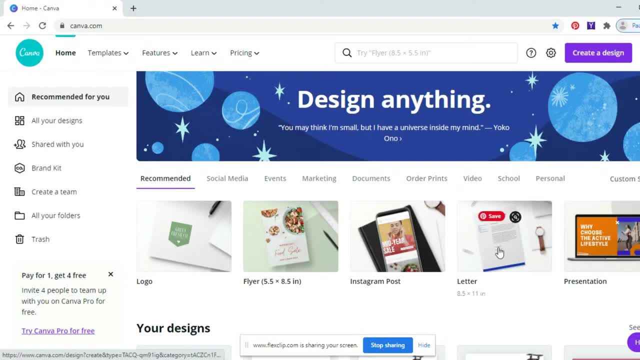 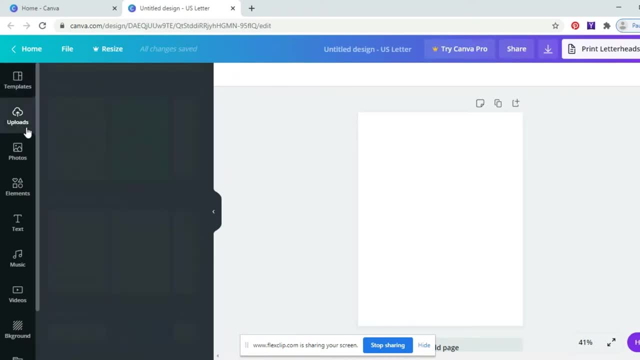 person in my list And then did that until I finished all of my character cards. Now that all my character cards are done, I'm gonna go back into Canva and open up a new file and I'm gonna make this one a letter size, because that's just a standard sheet of paper printing size. 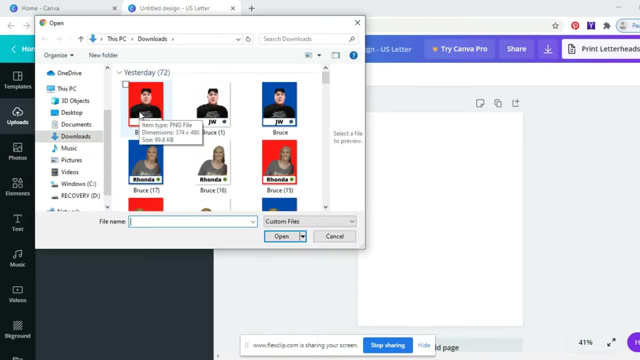 And so I'm going to put all of my cards, or as many as I can, on a sheet, because, since they are all individual images, it would be hard to print one on each page. So I did go in here and I uploaded the images of my little people. 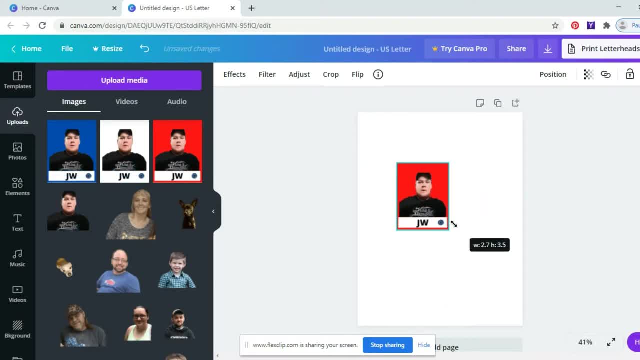 my little characters. I sized them down to the size I needed them to be, which was the 1.25 by 1.6., And then I just put as many of these little people character cards- onto a sheet as I could fit. 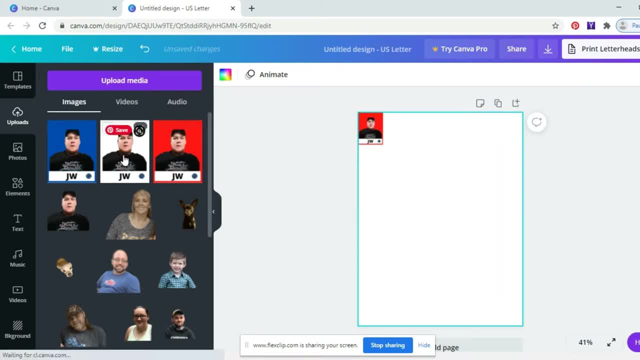 I ended up having to use two sheets to fit everyone on them, but I just individually, one at a time, put each image on Here and until I filled up the sheet at first, you can see I'm putting the white images on here to the white cards. 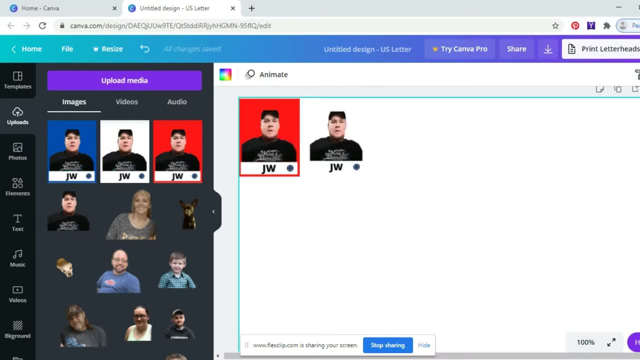 but I later changed my mind and decided to just do all of the red and blue cards on one sheet together and then to put all the white cards on a sheet together, And I made the white cards just slightly bigger. I made them about two inches instead of 1.6 inches. 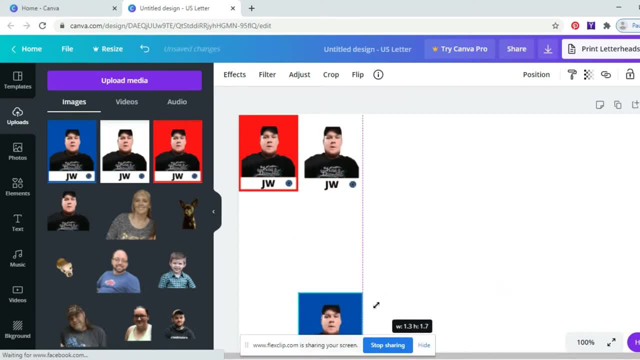 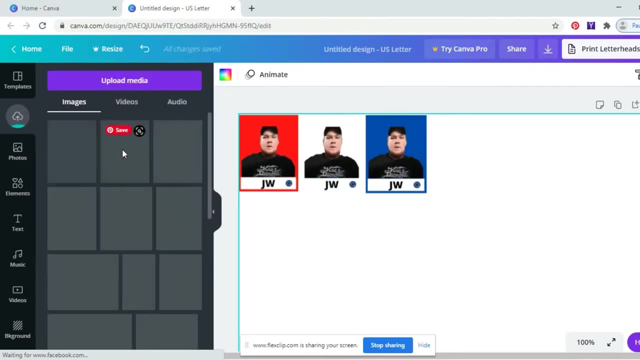 Again, this could all vary based on how big of a slot you have in your board pieces to put your pictures. So I'm just going to go down the line and add the images of everyone that I have for the game. My game required me to have. 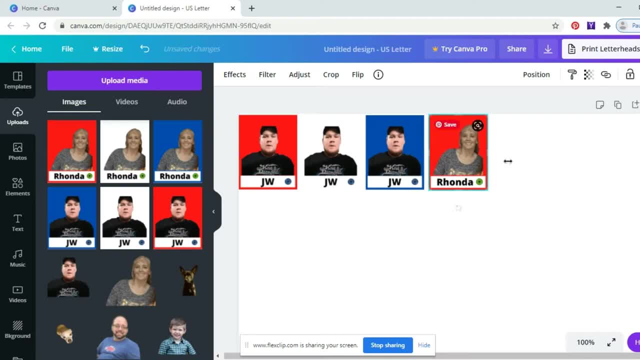 I think it was 24 people, I did. I did actually run out of people and have to put a couple of dogs on this game, just because I kind of wanted it to just be like super close people that we know enough about that we could do the questions for. 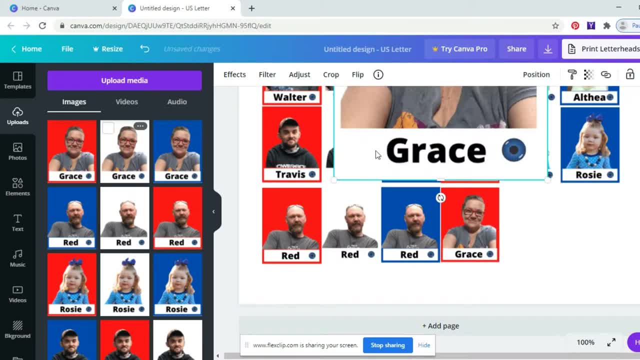 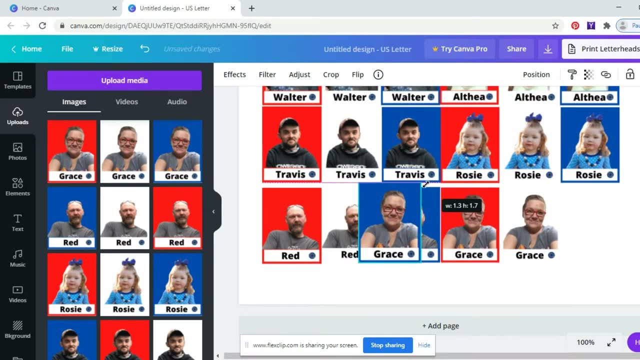 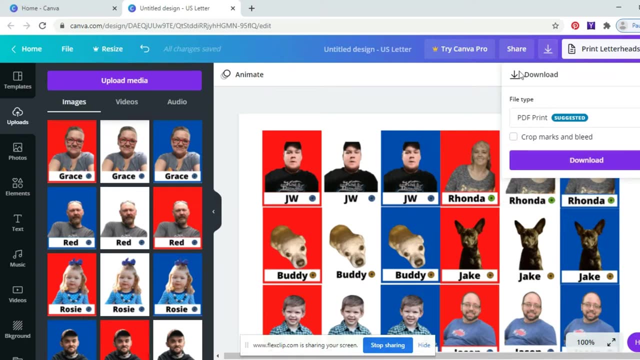 And I just ran out of people, So I ended up doing dogs. I do save this file as a PDF. The reason I do that do that is so they keep their size when I'm printing them. Once you get all of this done with all of your 24 people, 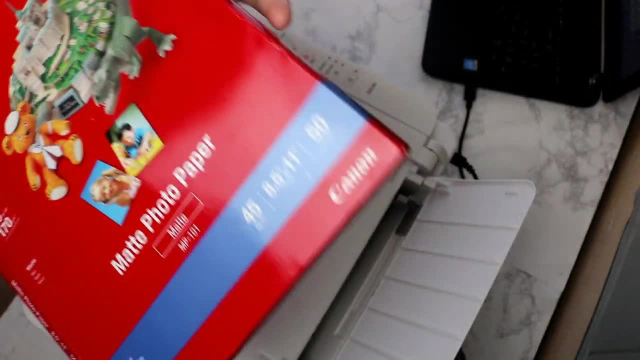 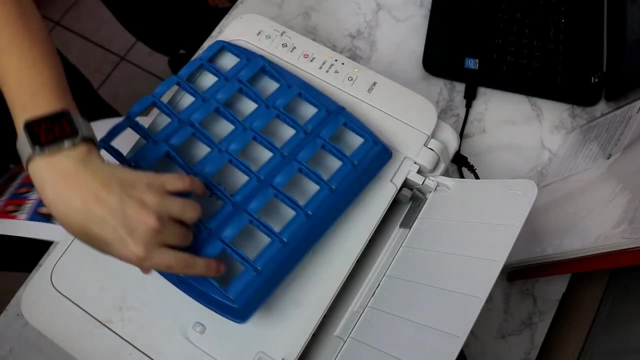 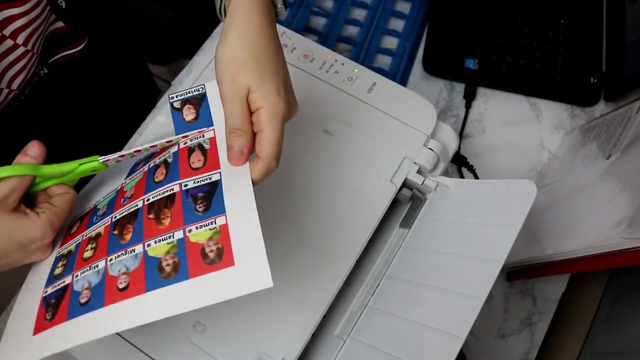 three images per person. I'm going to print these on photo paper because it's just a little bit sturdier than regular paper And I did not have cardstock, So I did print these out on photo paper. I slowly cut out the pictures, just so I can make them as straight and clean as possible. 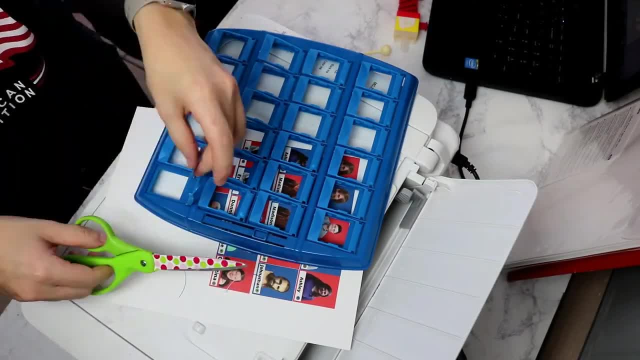 I checked my board to see if they would fit. It was a little bit big so I just trimmed a little bit on the size. This until I was able to get it to fit. So I did have to trim all of the pictures on the sides. 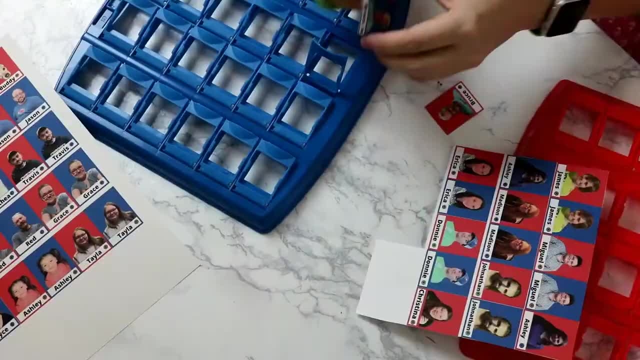 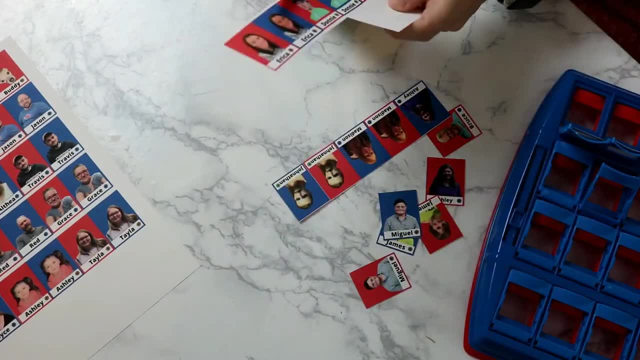 It didn't end up cutting off any of the pictures, so it all worked out. So I just go down the line through all of my pictures and cut them all out, one at a time. I cut them out very slowly. You just can't tell, because I have this fast forwarded like super fast. 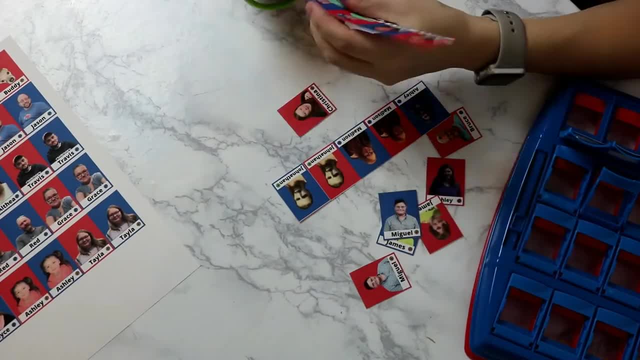 but I did try to take my time and be careful cutting out the images. As you can see, I did all the blue and red on one sheet and I did all of the white on a separate sheet, so I can make them a little bit larger. 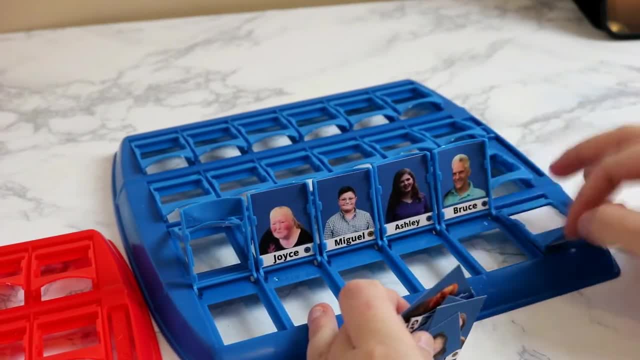 So now I'm going to take all of the pictures with the blue backgrounds. There's me And I'm going to just slide them in. I'm going to slide them in, Slide them into the blue board, not in any particular order. 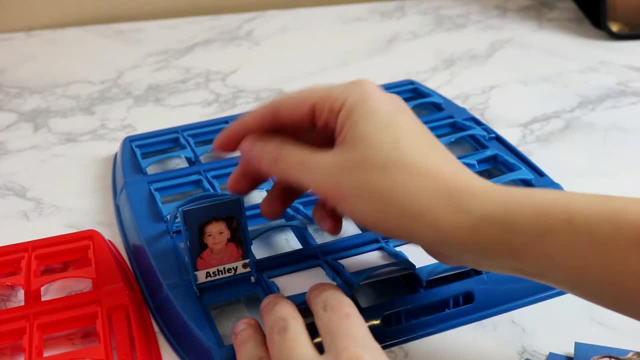 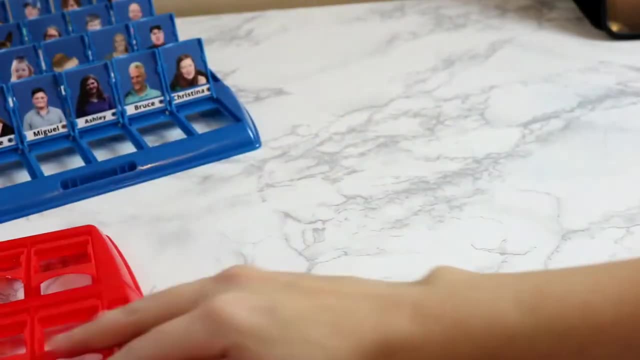 I'm just going to kind of cram them in any random way, because I kind of didn't want them to be predictable where they were. So I just randomly picked up cards and shoved them in wherever they went. again, with the red board I did the same. 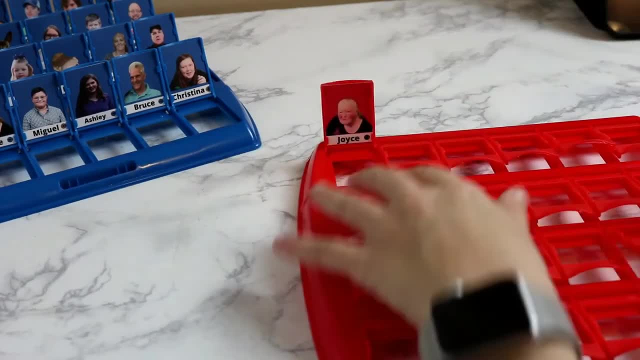 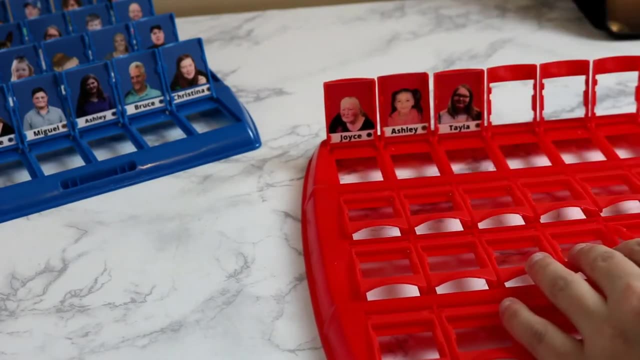 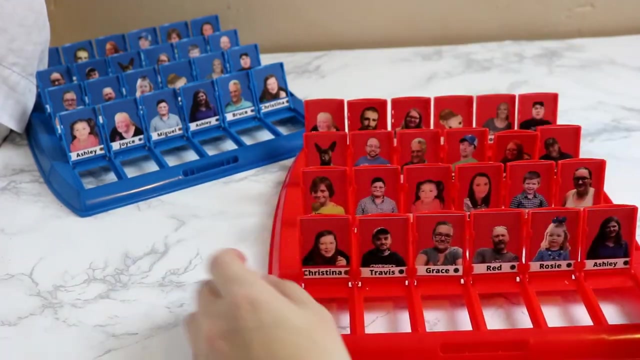 I got all of the cards that I made with the red background and I put them in the slots until I filled up the entire game board. Once your game board is completely filled up, it is time to work on the pictures that will go in the front that you're going to draw out of, and I just cut them out again, carefully and slowly. 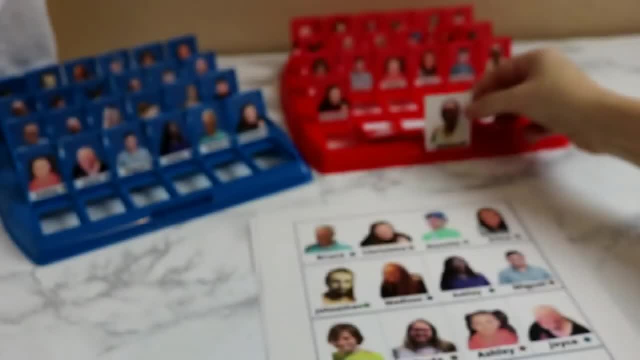 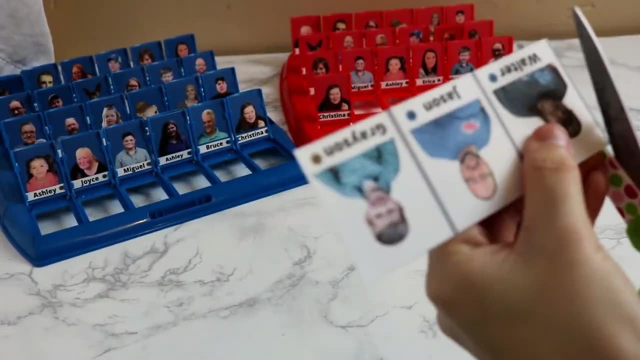 I did use the elements and the shape option to put a large gray rectangle behind all of the white cards and I spaced them out enough that I could see the gray lines between, so I would know exactly where to cut these out. I forgot to mention that because I didn't record it. 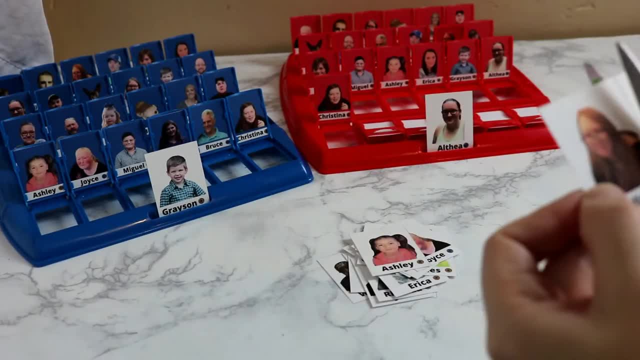 I didn't record when I redone the cards, But yeah, And once you get all of these cut out, you're pretty much ready to play your game. These are the ones you draw your character or who your person is going to be guessing. 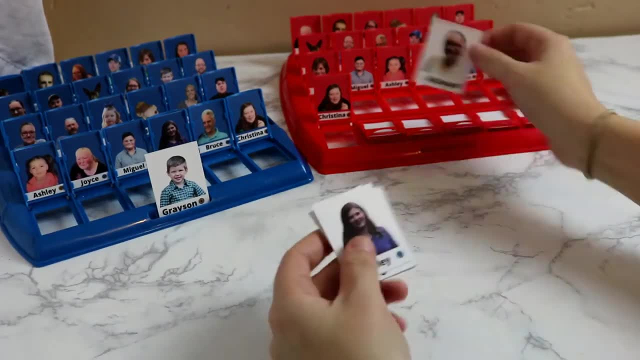 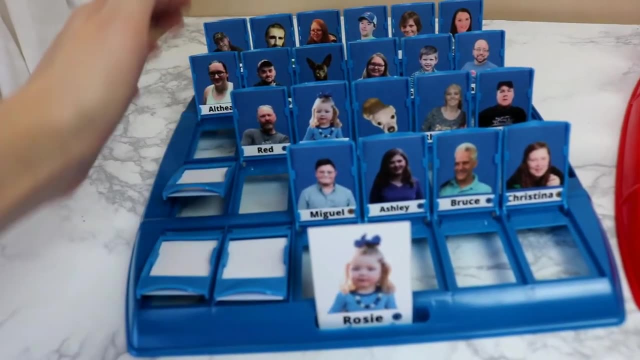 And that's it. After that, you just play the typical rules and game of guess who, as you would if it was just a regular store bought game. Only, it's so much funner because you have all your personal friends and family to make it interesting. 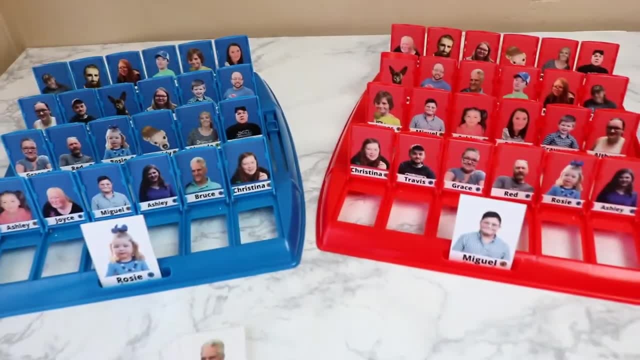 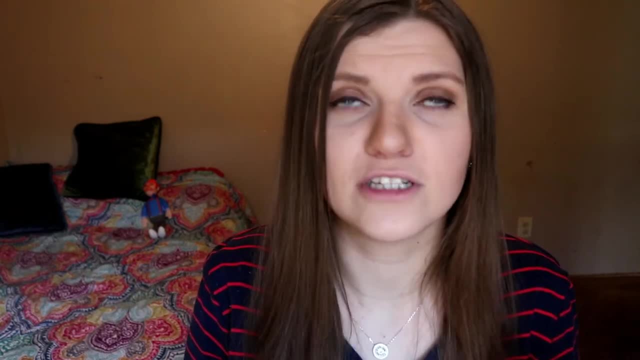 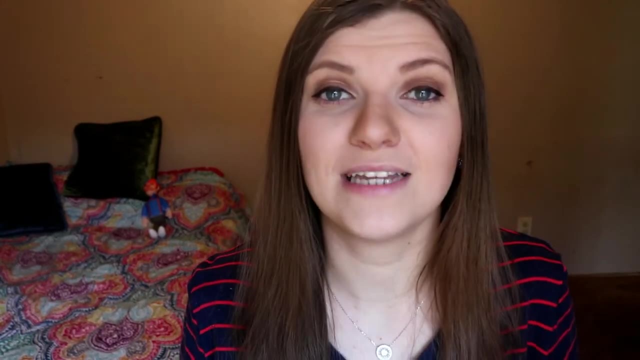 I cannot stress to you how fun this game is. So my husband's never played guess who and I feel so bad for him Because guess who was one of my favorites as a kid. So when I got this idea I knew I had to run with it, and I'm so glad I did because it turned out so cute. 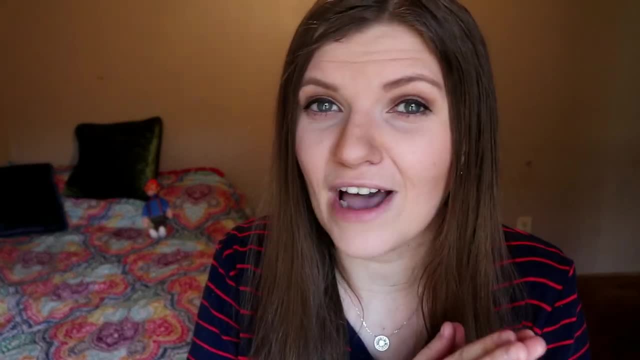 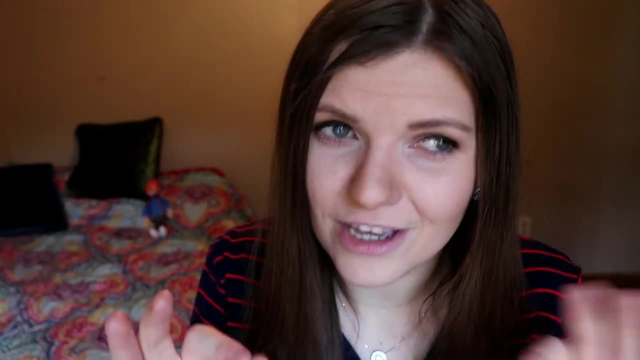 I actually got my guess who board at the dollar store for five dollars. I highly suggest you just go buy the actual guess who boards The dollar store. ones are made really cheap. They don't flip down really good, Just pay the extra few dollars. 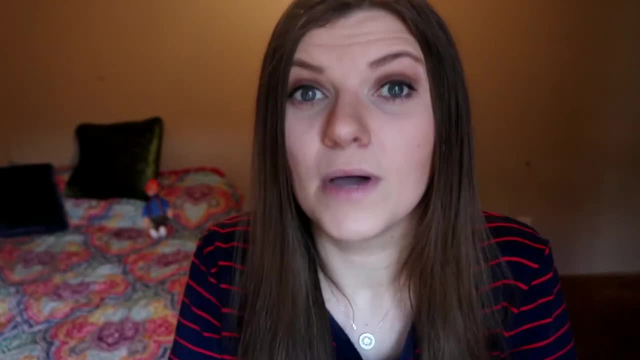 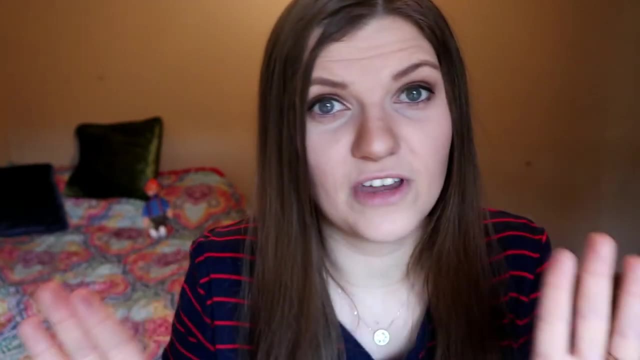 Go to Walmart and get you the actual guess who board. But keep in mind that your measurements and all that will depend on your board If you're using a different brand board. all my measurements fit my board. That doesn't mean they'll fit a guess who board. 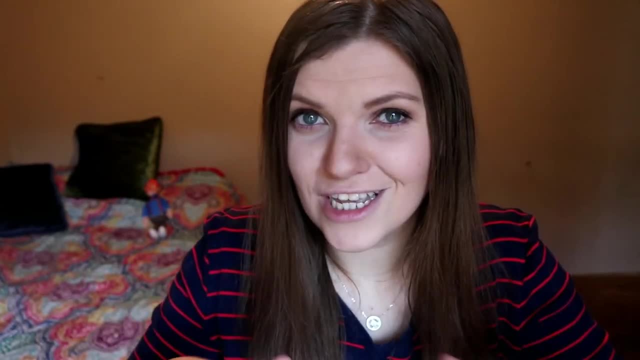 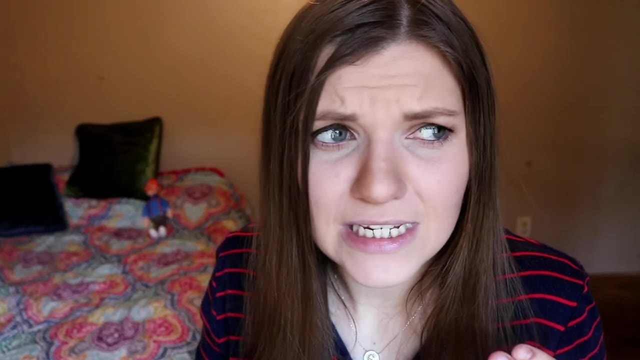 So when you're doing this, make sure you already have the game first So you can get all your measurements from it. Keep that in mind. But again, I do highly suggest: do not get the one I got Got. Do not get the one I got. 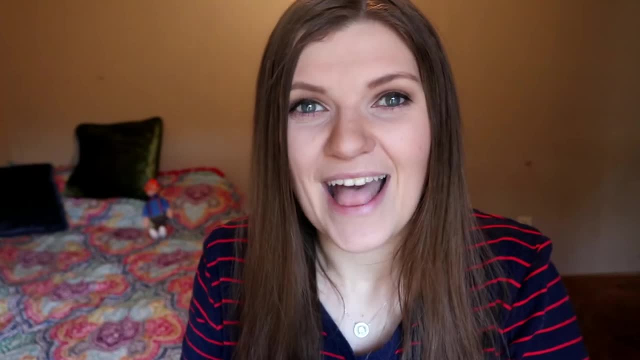 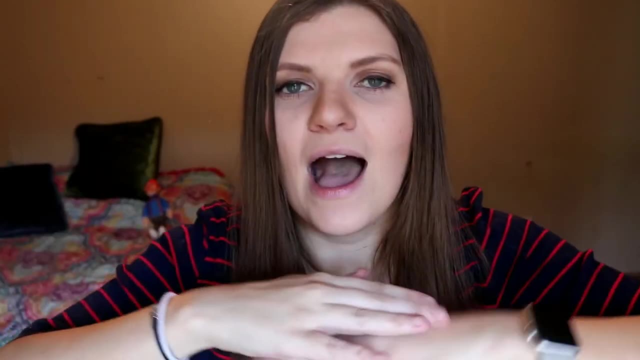 Get the guess who from Walmart. But with that said, I hope you like this video. I hope you guys like this guess who game. Leave a comment down below. Let me know what is your favorite board game. I love board games. I plan to make a ton more custom board games.